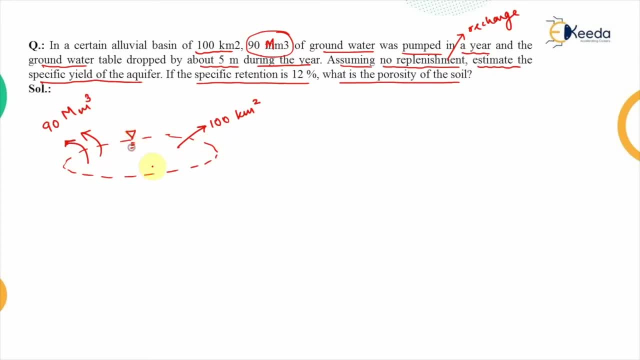 which this: if let's say this was the groundwater table, then it has dropped down by 5 meter during the year. That means this was the volume of the medium which was drained, because in the groundwater it is not possible that you are having only the water. The water is present within the voids of the 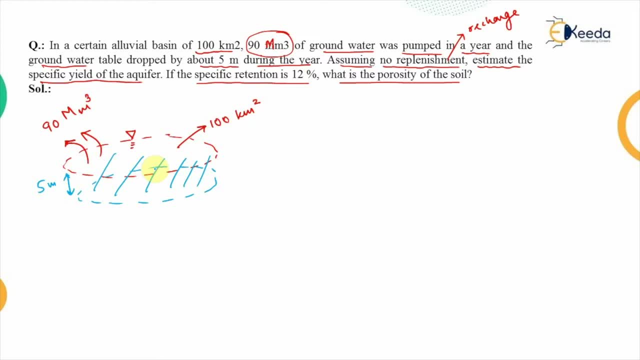 medium, So the height of the water table. when it has dropped by 5 meter, that means corresponding to the medium, the level has decreased. So this is the volume of the medium which was drained. Level has fallen about by about 5 meter. that means this will be the total volume which is being 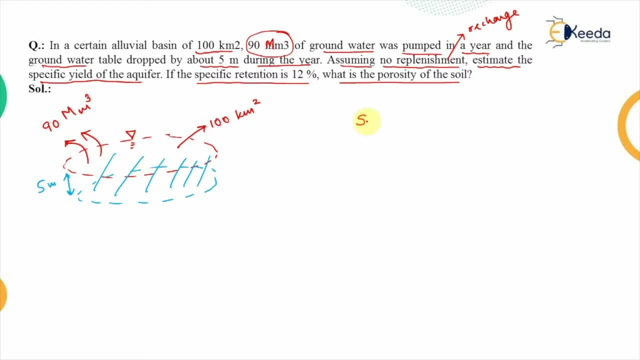 drained out. So we have seen that the specific yield is the volume of the water which is taken out. So the volume of water which is pumped out divided by the total volume of the medium from which this was taken out. So the volume of the water which was pumped out, that is. 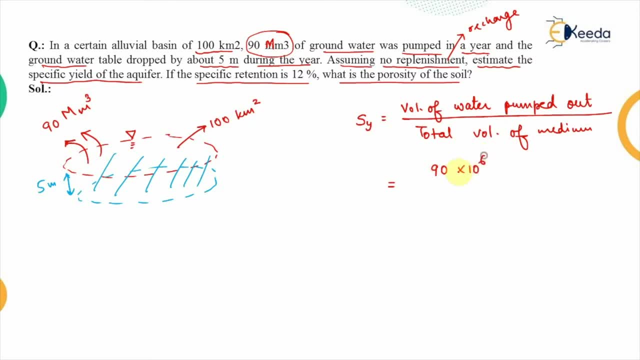 90 million cubic meter. So that will be 90 into 10 raised to the power: 6 cubic meter divided by the total volume of the aquifer, that is 100 square kilometer. So converting it into meter. So from here this 10 raised to the power 6 will be cancelled out. So specific yield is 0.18 and we 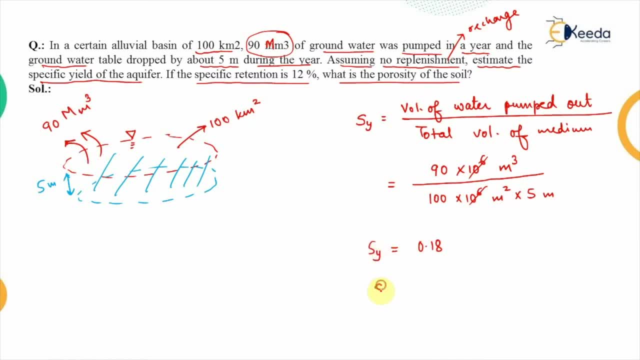 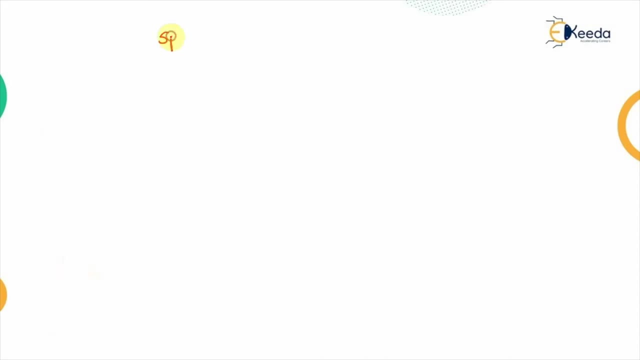 can also represent it within the percentage, that is, the specific yield of the soil is 18 percent. Now one more data is given. that is corresponding to the volume of the water. So this is the volume of the water which is taken out. So this is the volume of the water which is taken out. So this is the volume of the water which is taken out. 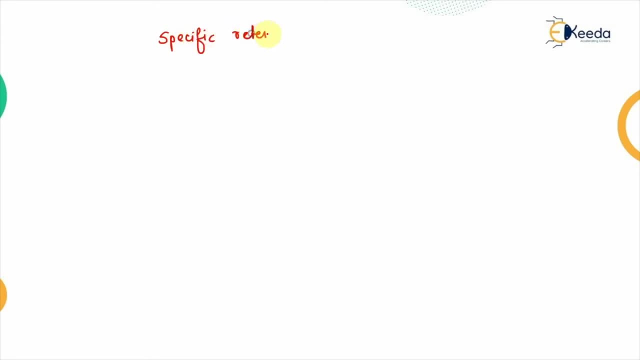 To the specific retention. that means against the gravity. that means against the gravity, what amount of the total medium was able to restrain against the flow, So that volume is given as that value is given as 12 percent. So if we club both the values that the specific yield, that is 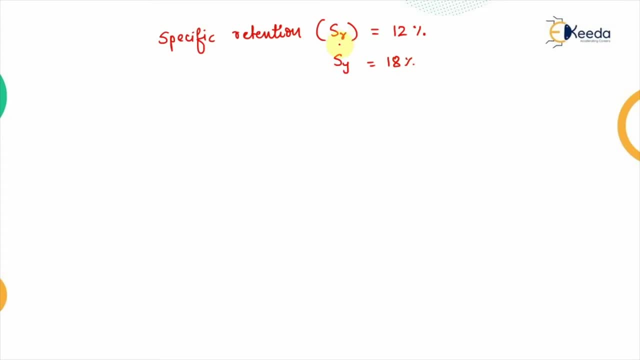 18% and the specific retention that is 12%. So if we take the entire volume, so let's say these are the medium particles which are arranged randomly now within the voids. only the water is present. Now either the water will be taken out or will not be taken out. The amount which 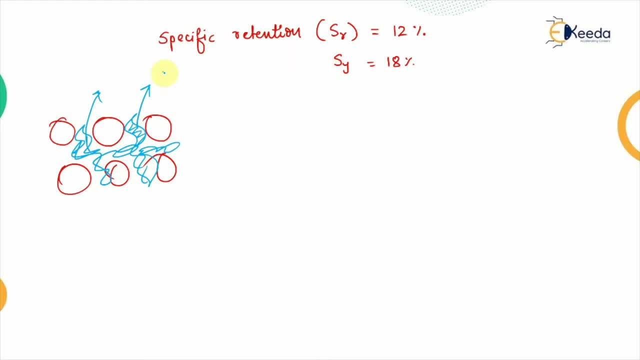 is taken out, that is given by specific yield, and the amount which is retained, that is given by specific retention. But if we add up both these values, that is giving us the volume of the voids, that for the total medium, in how much volume the voids are present, And 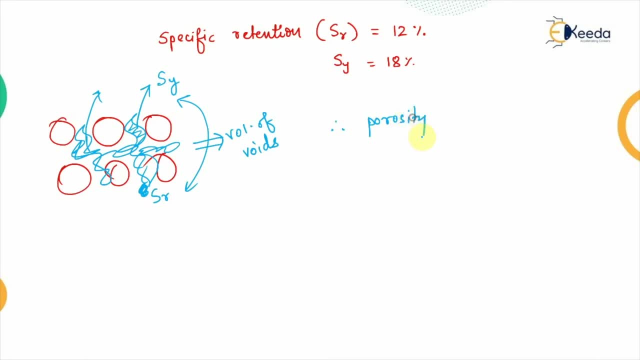 therefore, that volume of voids are represented by the amount which is taken out Now if we add the number of voids that are present, and that is represented by the porosity of the medium. So the porosity of the soil that is given by eta, that is equal to the Sr that 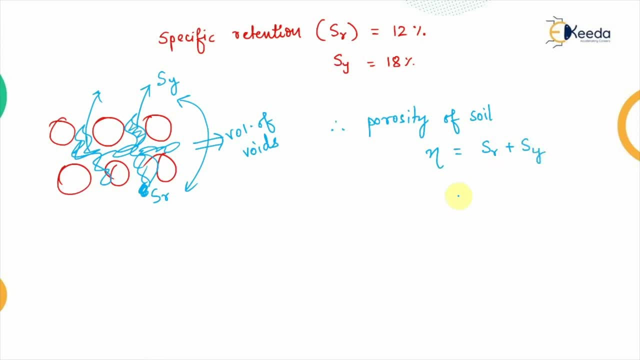 is the specific retention plus specific yield, so that will be 12% plus 18%. So the porosity of the soil, that is 30%. So that is the first problem that we have to do. so the first problem to solve is how to solve it. The first problem to solve is the problem that we have to solve. 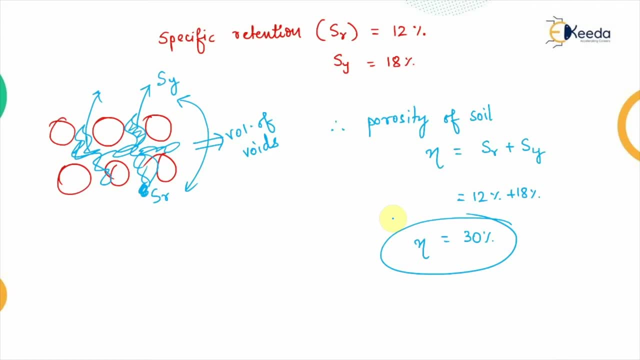 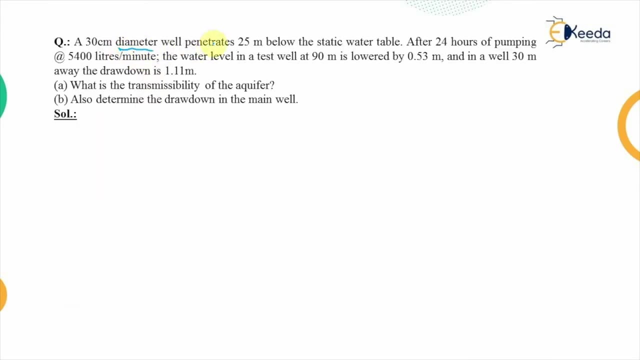 was discussed, to calculate the porosity of the soil. The next problem is it says that a 30 cm diameter well it penetrates 25 m below the static water table. Again, the steady conditions are given. that means they are corresponding to the theme's. 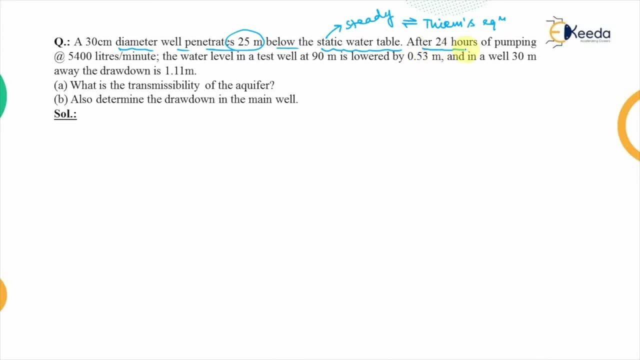 equation: After 24 hours of pumping, which is done at the rate of 5400 liters per minute, the water level in the test well at 90 m depth was lowered by. at 90 m, distance was lowered by 0.53 m and in a well which is 30 m away, it was: 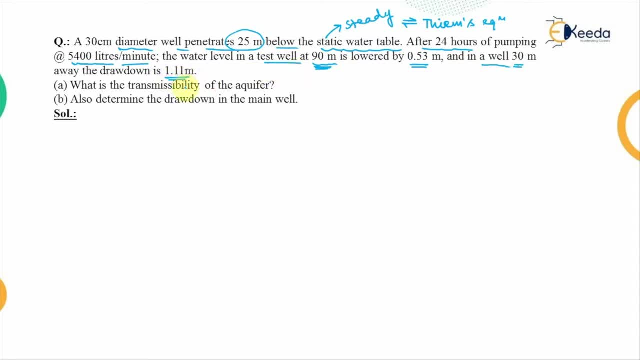 lowered by 1.11 m. Now here we have to calculate another factor that is known as the transmissibility of the aquifer, which is the coefficient of permeability into the width of the aquifer. In the second part we have to determine the drawdown in the main. well, Now this problem. 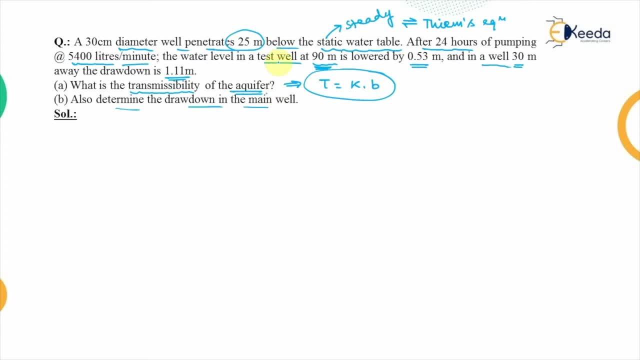 has been asked in the engineering services exam. Since the well is speenetrating 25 m below the static water table, it is evident that it is a case of the unconfined aquifer, because if this wasn't, then the well won't have. 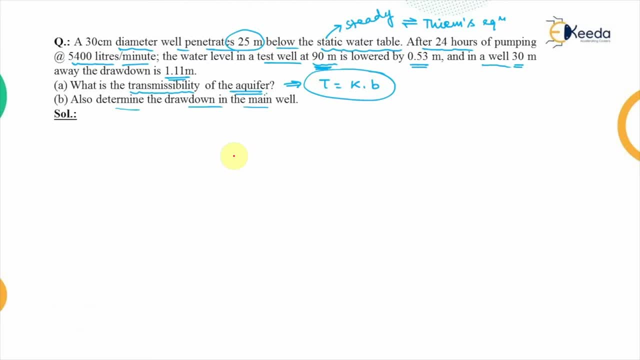 gone upto such depth, So the theme's equation for the discharge will be applied. that is given as, as q is equal to pi, k into h2 square minus h1 square divided by 2.303 log base 10, r2 upon r1.. 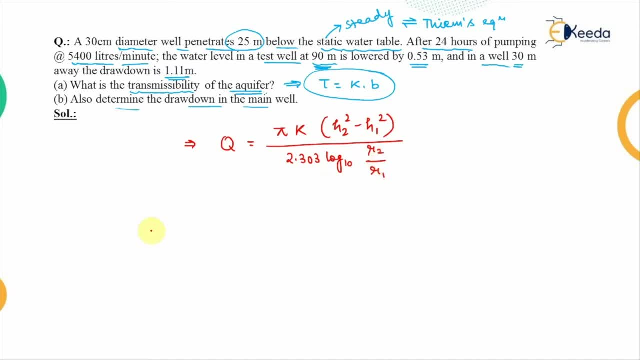 Now, one by one, we will calculate all the data. So corresponding to the second drawdown. if we look at the themes equation, this is the main pumping well Now corresponding to this: if water table has fallen down from this to this existing level, this will be the drawdown. 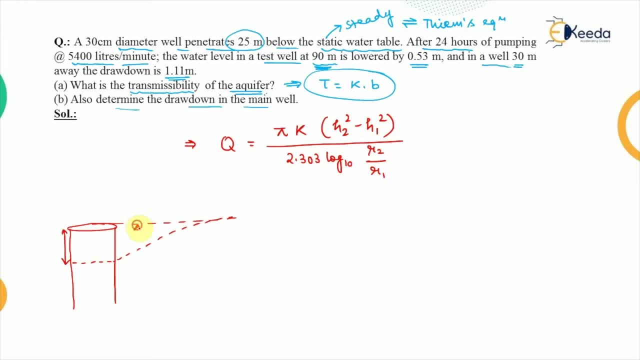 influence. At one location, which is 30 meter away, the drawdown is 1.11 meter. At another location, this is 0.53 meter. Now, this is at a distance of 30 meter and this is at a distance of 90. 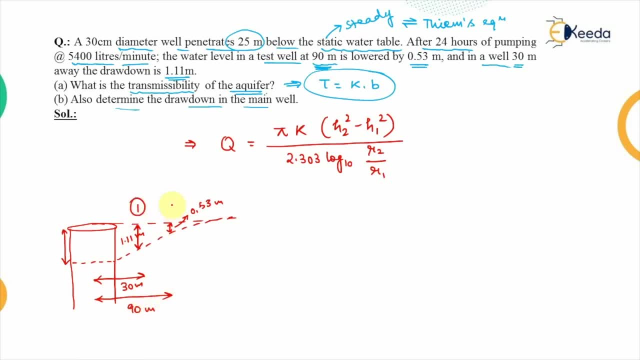 meter. So we are considering this as the first one and this is as the second one. So for first well, the drawdown that is given by s1, that is, is equal to 1.11 meter. Therefore, the value of the height of well, that is h1. that is d minus s1. total depth, that was 25. 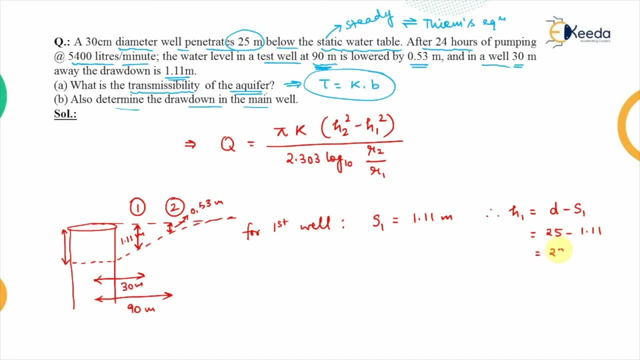 minus 1.11, this will be equal to 23.89 meter. Corresponding to first one, the radius is 30 meter. Now for the second. well, they drawdown that was given as 0.53 meter. therefore, h2 will be equal to d minus h2, that is, 25 minus 0.53. 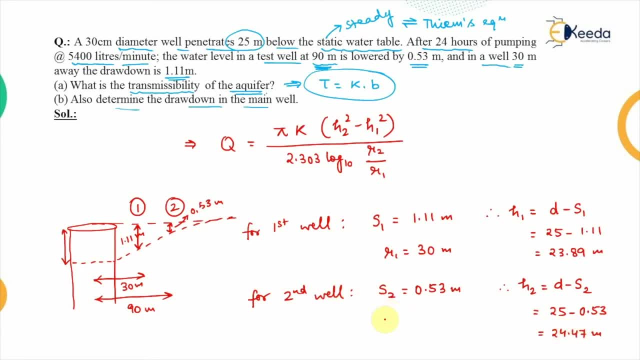 that is 24.47 meter. corresponding to this, the r2 value is 90 meters. now, this is the entire values that has been given now for both the cases. this pumping rate that was as 5400 liters per minute, now, since q value is given as 5400 liters per minute. 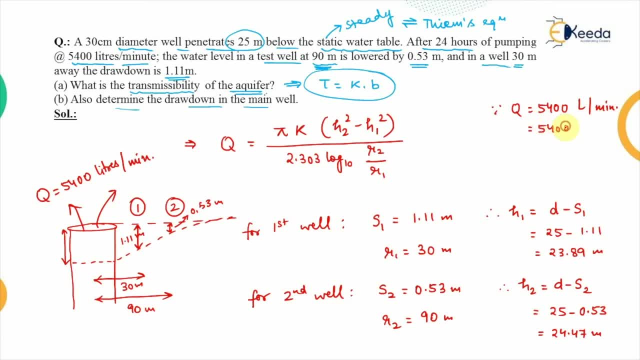 converting it into the standard unit, that is 54, into 10, raised to the power, minus d, minus h2, that is 24.47 meter. corresponding to this, the r2 value is 90 meters minus 3 cubic meter divided by 60 seconds. so from here this will be: 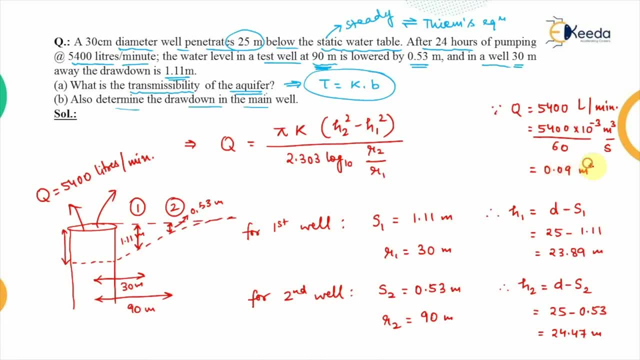 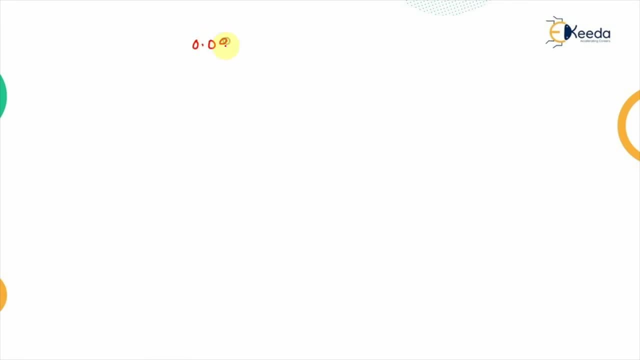 0.09 cubic meter per second. this will be the value of the discharge. now, substituting these values in the given equation by the theme, so placing the value of the q, that is 0.09, that is, is a equal to pi- into k, into, for the first case, this is 24.47 square, that is, h2 square minus h1 square. 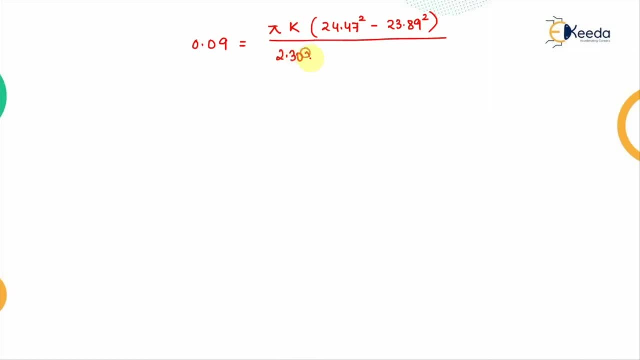 divided by this will be 2.303. log base 10: r2 is 90. divided by r1 is 30.. so from this, if we can calculate the value of the coefficient of permeability, that is 0.09, into 2.303. 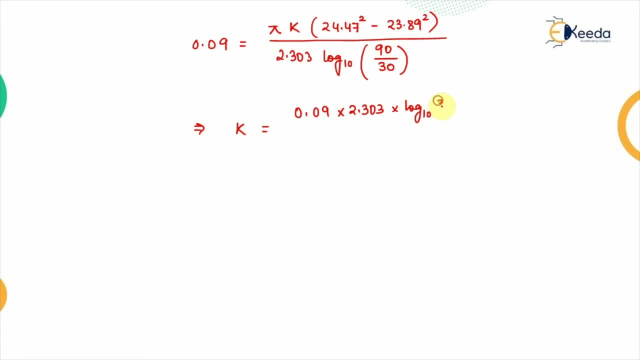 into log base 10: 90 upon 30, that is 3. divided by this value is 3.14 into 24.47. that is a square minus b square. from here, if we calculate the value of this coefficient of permeability, that comes out: 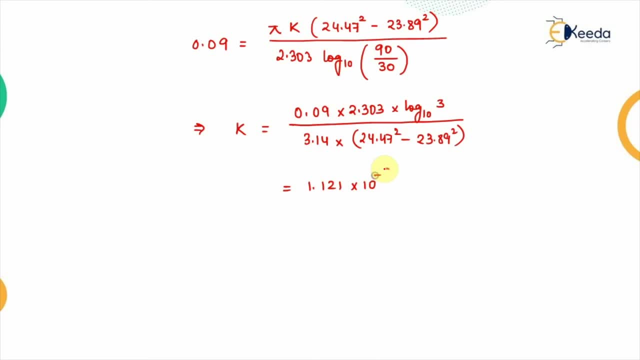 to be 1.121 into 10, raised to the power minus 3 in the units of meter per second. that is the coefficient of permeability. Now, therefore, the transmissibility that is given by capital T, which is equal to k into b, or that is written as k into d. that is the width of the aquifer. 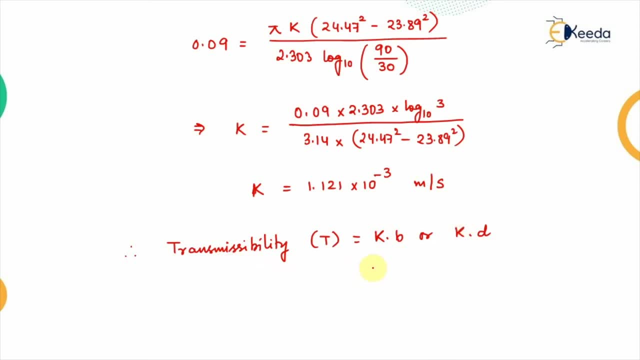 So here we are representing that value by the depth. So So this coefficient of permeability, that is 1.121, into 10, raised to the power minus 3 in meter per second, the value of d, that is 25.. So the units of the transmissibility will be square meter per second. 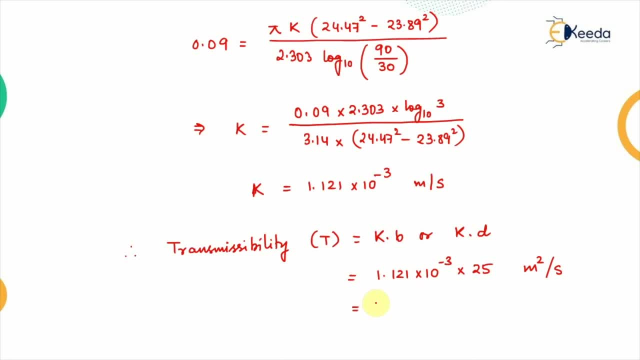 So from here, the answer that we are getting, that is, is equal to 0.028 square meter per second. Now, to have this value as the significant one, we can convert this into the minutes, So this will be: is equal to 1.68 square meter per minute. 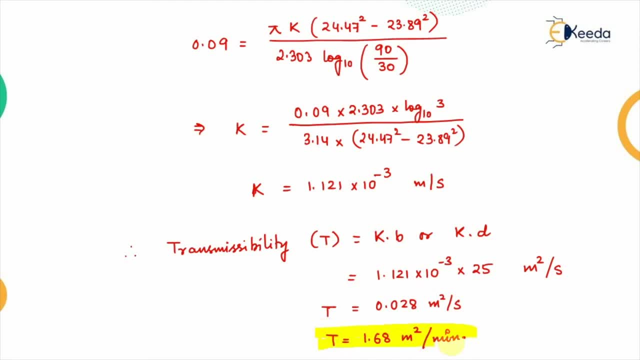 So this is the result, correspondingly To the transmissibility of the aquifer. that completes the first part of the problem. Now, in the next part, we have to calculate the drawdown in the main. well, So now we want to calculate the drawdown in the main. well, 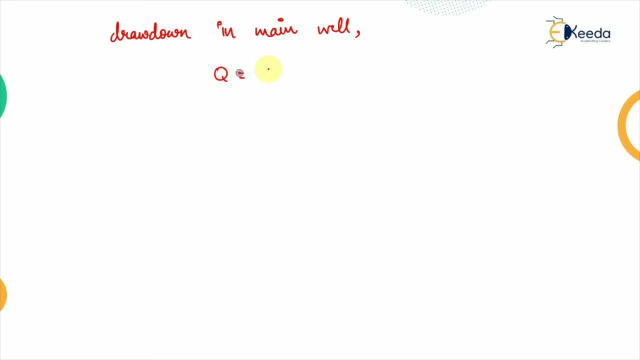 So to calculate this we will again use the same formula. that is done for the Unconfined aquifer, that is, pi into k, into h2 square minus h1 square divided by 2.303 log base 10, r2 upon r1.. 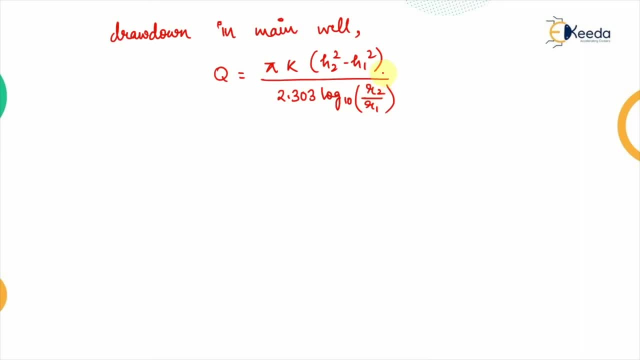 Here what we will do: in place of h2, we will use the h1, and in place of h1, we will use the hw, because what we are doing Now we want to calculate This drawdown level, that is for the main. well, so that is given as SW and the remaining height will be hw, corresponding to the first observation. well, this is S1, and remaining one is h1. 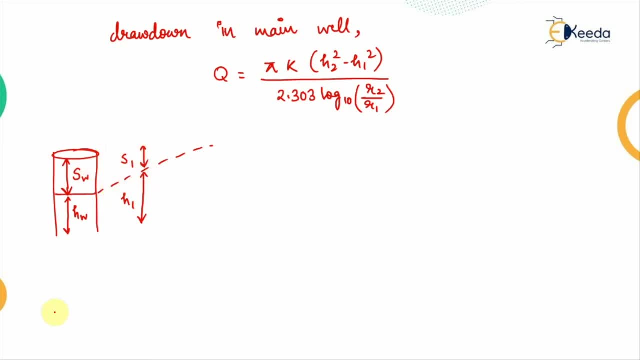 We will take these two data points only. So, in place of h2, we will use now h1, and corresponding to h1, we will use hw. So, in place of h2, we will use now h1, and corresponding to h1, we will use hw. 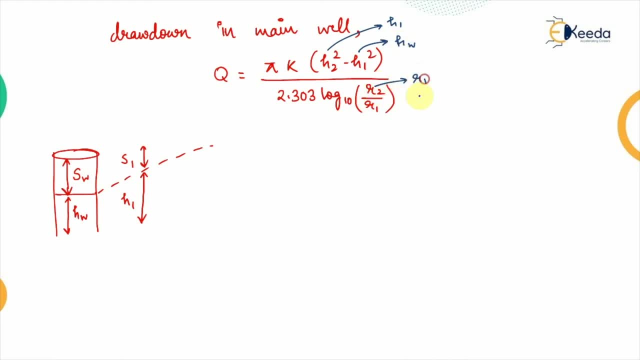 So in place of h1, we will use now hw. So corresponding to r2, this will be r1, and corresponding to r1, this will be the radius of the well. So since the discharge rate remains the same, so that is 0.09 cubic meter per second. 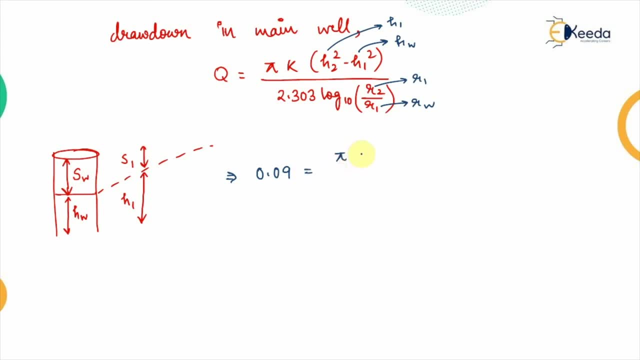 This pi value that remains the same, into this coefficient of permeability that is 1.121.. So in place of h2 we will use now hw 10, raised to the power minus 3 h2 square. now here this is h1 square. so first of all i'll write down: 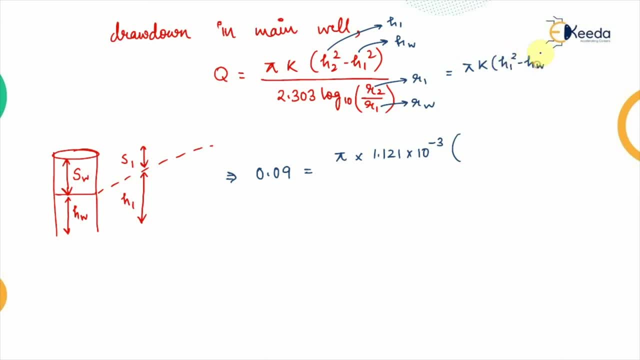 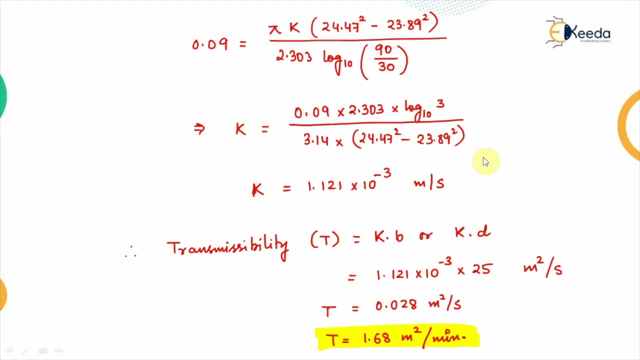 the changed formula, that is h1 square minus hw square, divided by 2.303 log base, 10 r1 upon rw, so h1 square so that will be equal to 23.89 square minus hw that we do not know. divided by 2.303 log base, 10 r1 is 30 meter, while the radius of the well that is given to us. so 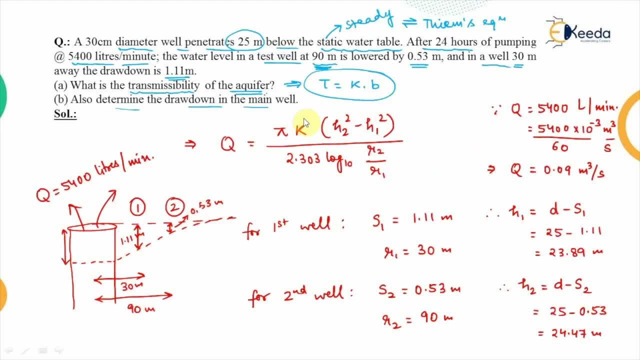 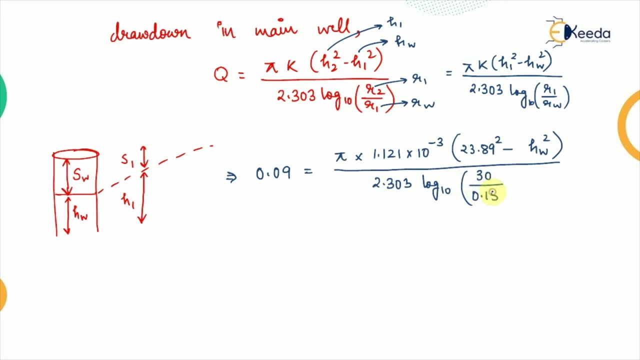 the diameter of the well. so that was given to us as 30 centimeter. this diameter was given as the first data point, so this value is 30 centimeter. so the radius will be 15 centimeter. so converting that into meter, this will be 0.15 meter radius of the well. that was 15 centimeter. converting that into meter is: 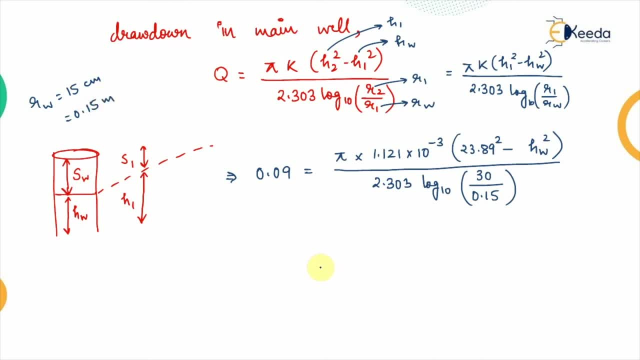 0.15. so so, so, so, so, so. so, corresponding to this drawdown, we will be getting the this drawdown, we will be getting the this drawdown lower than national radius of the influence and, correspondingly, we will be having the zone of influence. Now, that completes all the type of problems based on the. 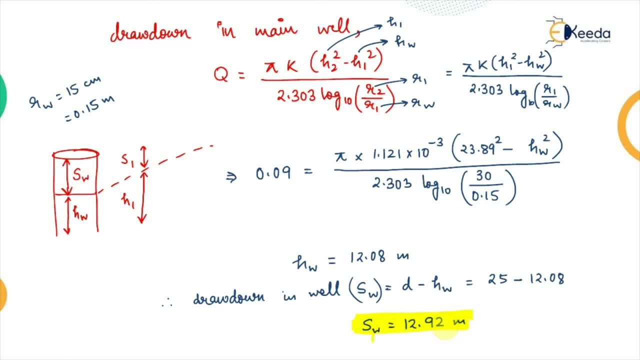 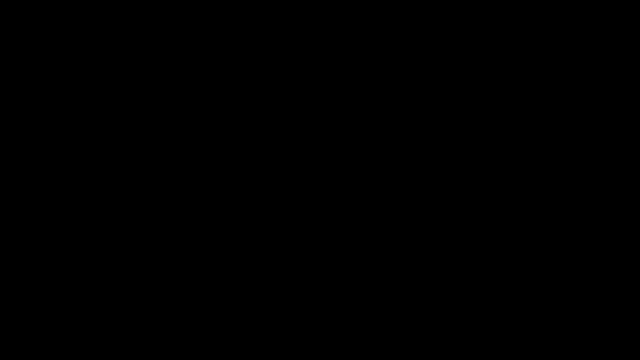 chapter of the groundwater. In the next video we will start the new chapter that is based on the reservoir planning. Thank you you.